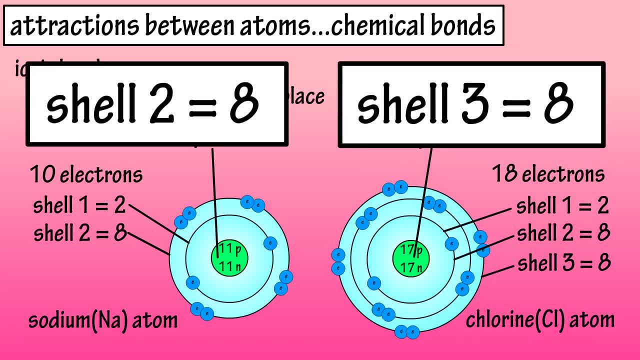 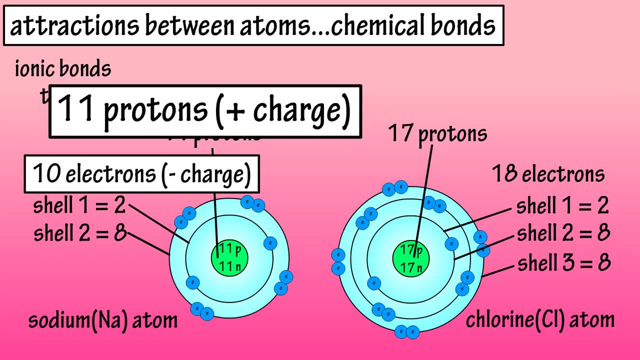 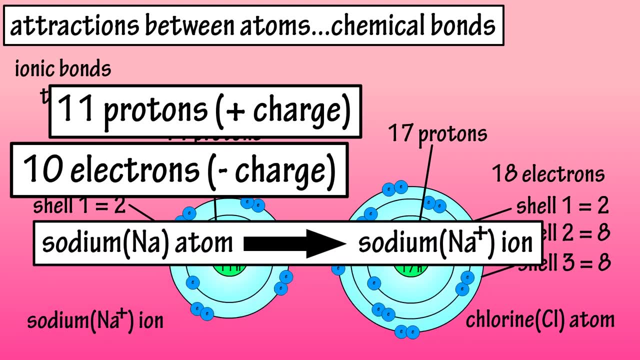 And that will give it eight electrons in its outer shell. Since the sodium atom gave up an electron, it has 11 protons which are positively charged and 10 electrons which are negatively charged. This results in the formation of a sodium ion with a positive charge. An ion is an atom or 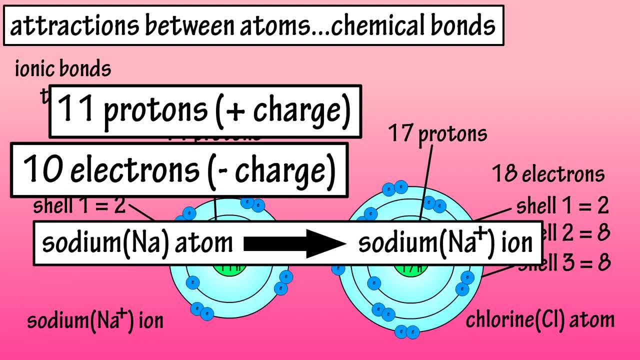 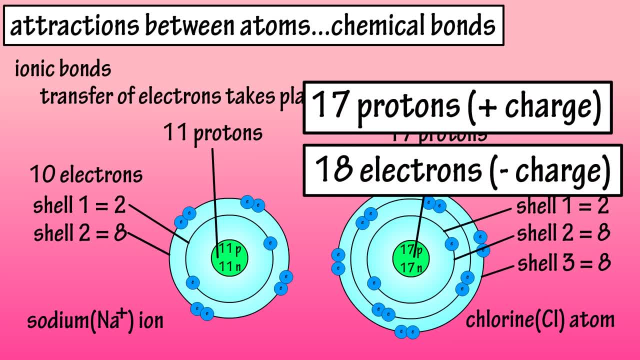 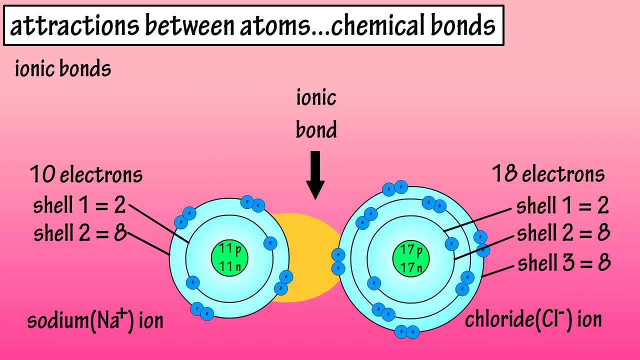 molecule with a net electrical charge due to the loss or gain of an electron. Since the chlorine atom gained an electron and now has 17 protons and 18 electrons, it has a positive charge. It is a chloride ion with a negative charge. The positively charged sodium ion is now attracted. 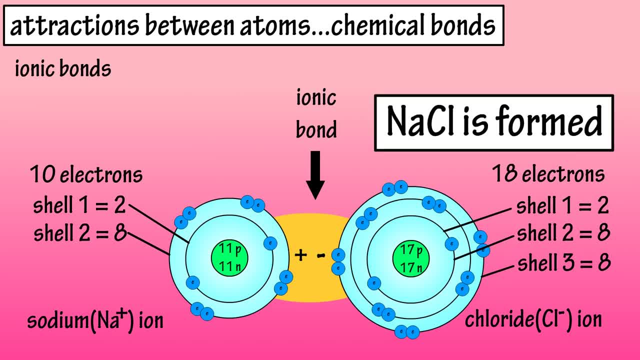 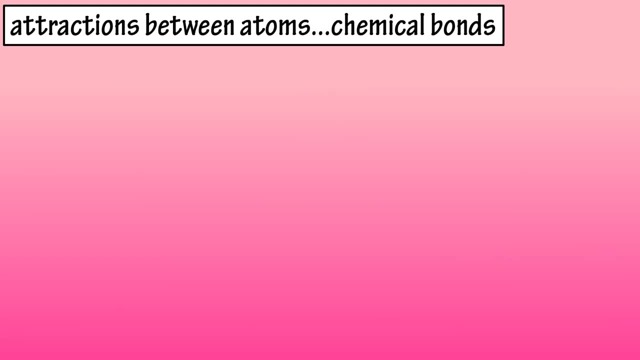 to the negatively charged chloride ion and NaCl or table salt is formed. This is an ionic bond. so ionic bonding is when an electron transfer takes place and generates two oppositely charged ions. Now for covalent bonds. Covalent bonds are chemical bonds that are formed by the sharing of 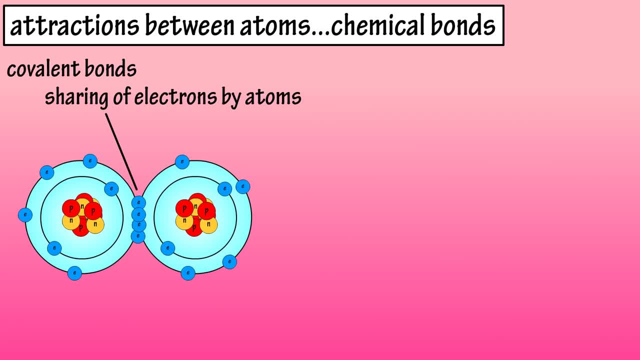 one or more pairs of electrons. The covalent bonds are the bonds that are formed by the sharing of electrons by the outer energy levels or shells of two atoms. The four major elements of the body- carbon, oxygen, hydrogen and nitrogen- almost always form covalent bonds by sharing electrons. 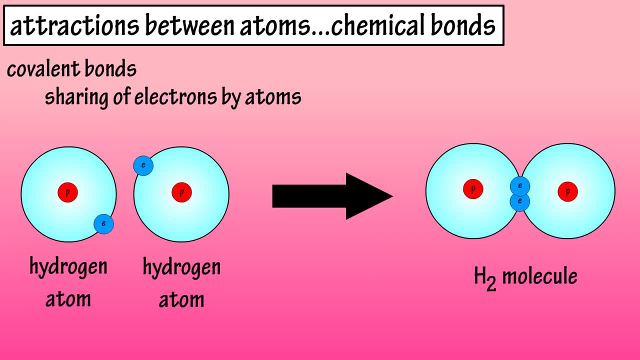 So, for instance, two hydrogen atoms can bond by sharing a pair of electrons. Hydrogen is one of the exceptions to the octet rule of having eight electrons in the outer shell, because it only has one shell. Let's look at carbon dioxide, or CO2, which forms a covalent bond. Oxygen has an atomic. 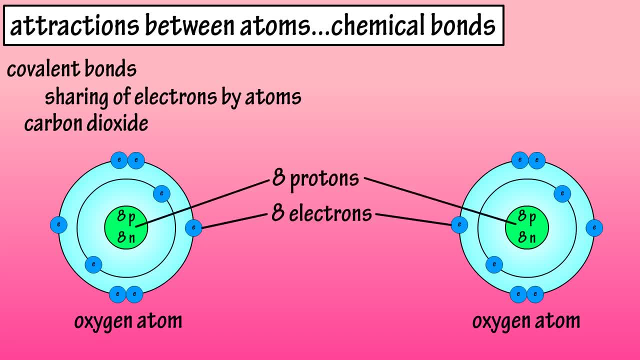 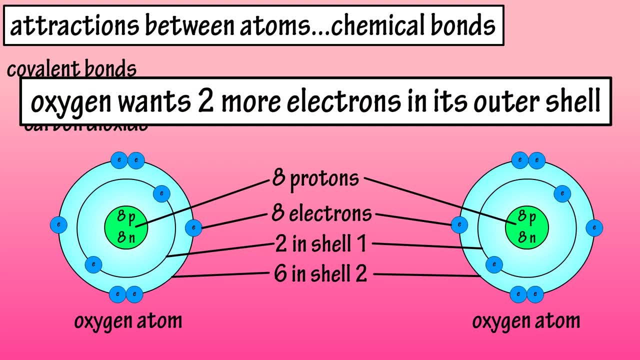 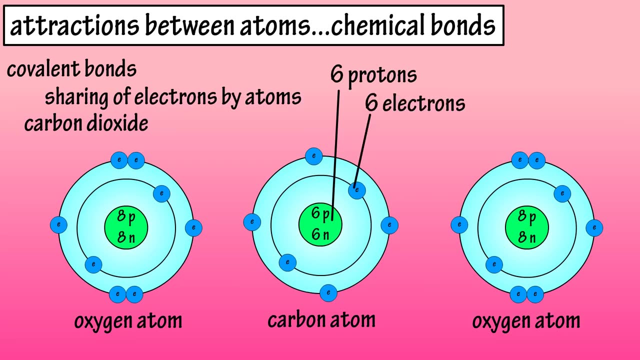 mass of eight. So eight protons and eight electrons. Two electrons in its inner shell and six in its outer shell. So oxygen atoms want two more electrons for their outer shell. Carbon has an atomic mass of six, Six protons and six electrons, Two in the inner shell and four in the outer shell. 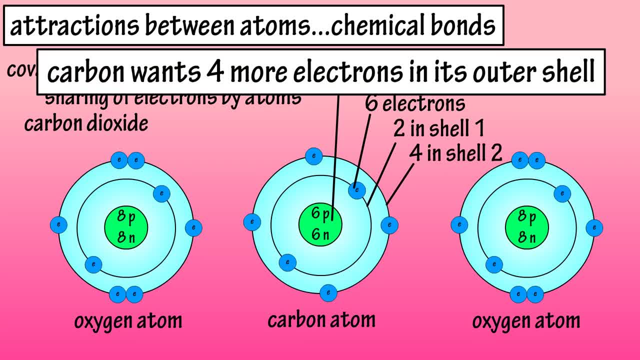 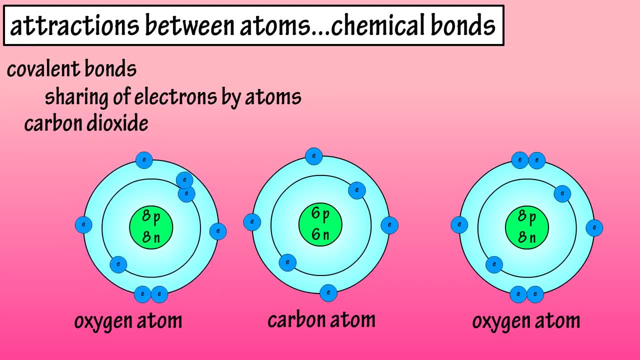 So it wants four more electrons for its outer shell. These fellows can make each other happy by sharing what they have. Oxygen atom number one can share two of its electrons with the carbon atom, and in return the carbon atom can share two of its own electrons with oxygen atom number one, making oxygen atom number one happy, Then oxygen.